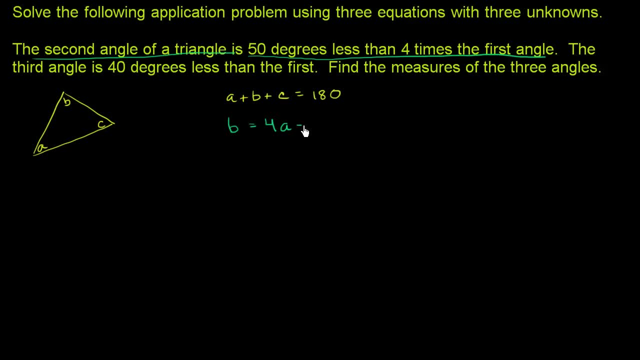 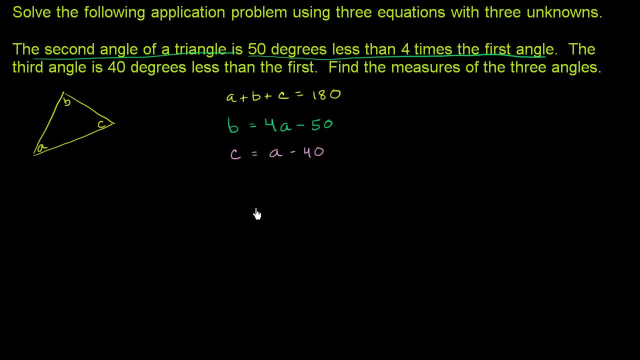 So the first angle is A and it's going to be 40 degrees less than that. So we have three equations with three unknowns, And so we just have to solve for it And let's see what's a good first variable to try to eliminate. 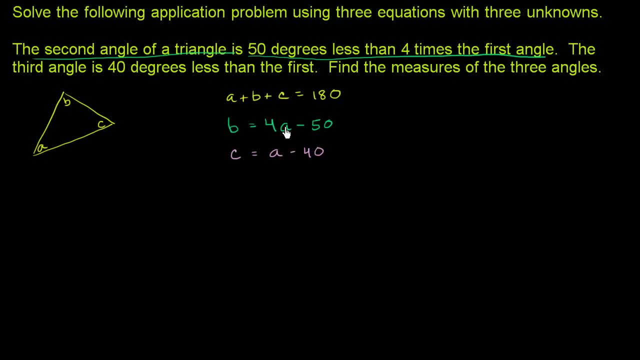 And just to try to visualize that a little bit better, I'm going to bring these A's onto the left-hand side of each of these equations over here. So I'm going to rewrite the first equation: We have A plus B plus C. 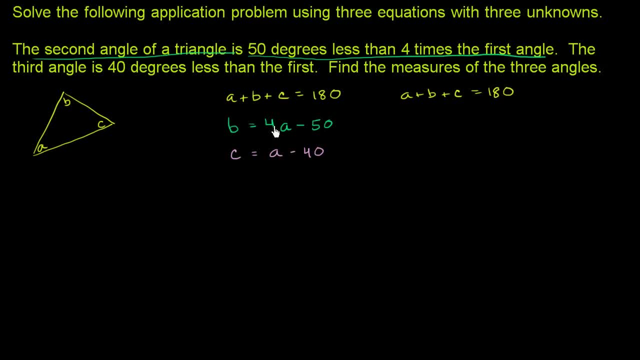 It's equal to 180.. And then this equation: if we subtract 4A, from both sides of this equation, if we subtract 4A, we have negative. 4A plus B is equal to negative 50.. And then this equation, right over here: 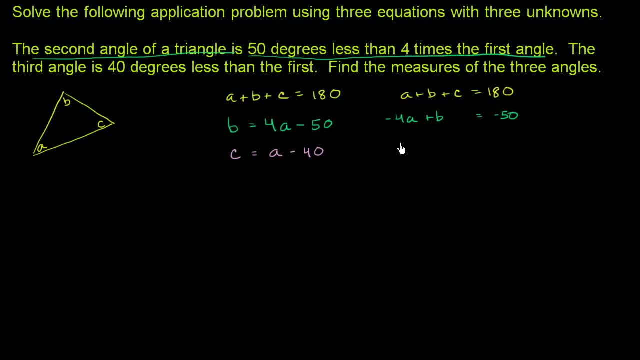 if we subtract A from both sides, we get negative A plus C. Negative A plus C is equal to negative 40. I just subtracted A from both sides. So we now want to eliminate variables And we already have this third equation here. 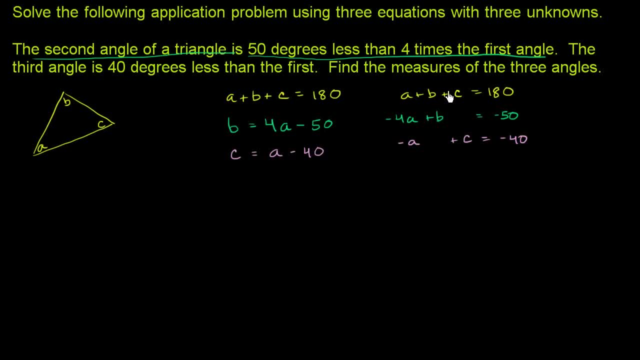 is only in terms of A and C. This is only in terms of A and B, And this first one is in terms of A, B and C. So if we could, let's see, this is already in terms of A and C. 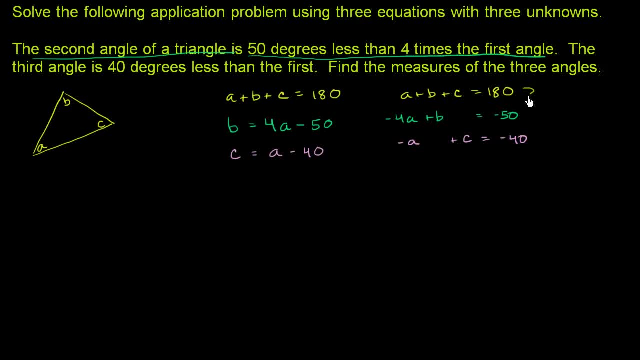 If we could turn these first two equations, if we can use the information in these first two equations to end up with an equation that's only in terms of A and C, Then we could use whatever we end up with along with this third equation right over here. 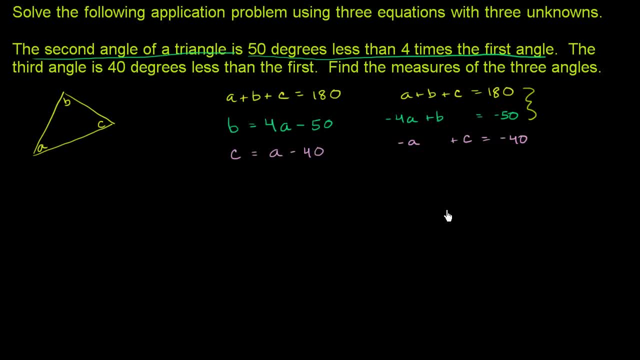 And we'll have a system of two equations with two unknowns. So let's do that. So if we wanted to just end up with an equation only in terms of A and C, using these first two, we would want to eliminate the B's. 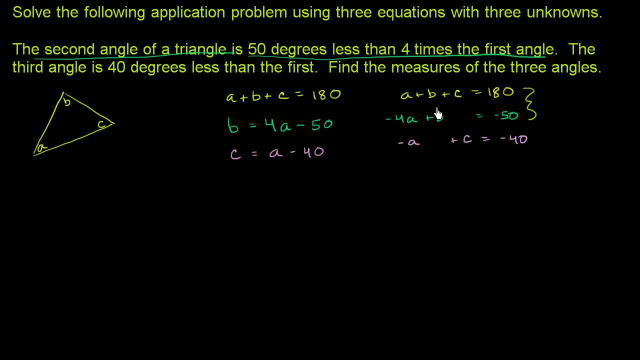 So we could multiply one of these equations times negative 1, and one of these positive B's would turn into a negative B. So let's do that. Let's multiply this first equation over here. Let's multiply it times negative 1.. 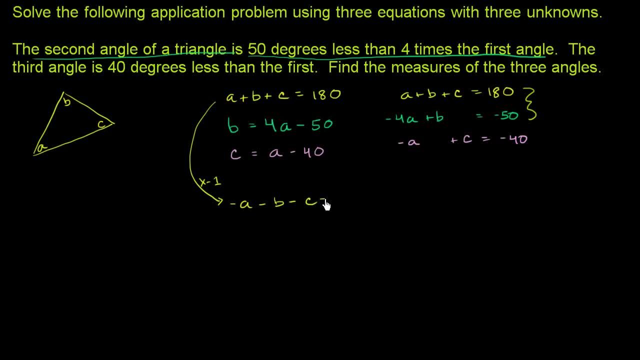 So it'll become negative A Minus B minus C is equal to negative 180.. And then we have this green equation right over here, which is really just this equation just rearranged. So we have negative 4A plus B is equal to negative 50.. 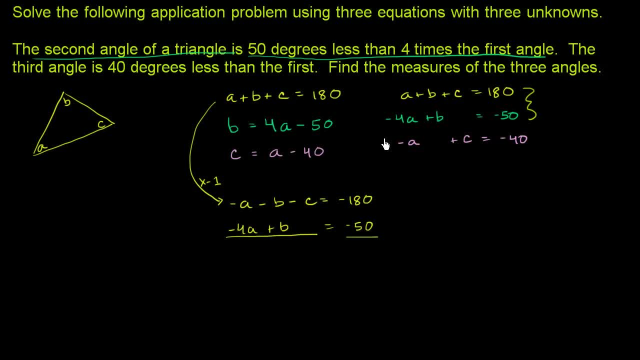 And now we can add these two equations. I actually should have done that in a. actually, let me do that in the other color, just so you see where that's coming from. Do it in that green color. So this is negative 4A plus B. 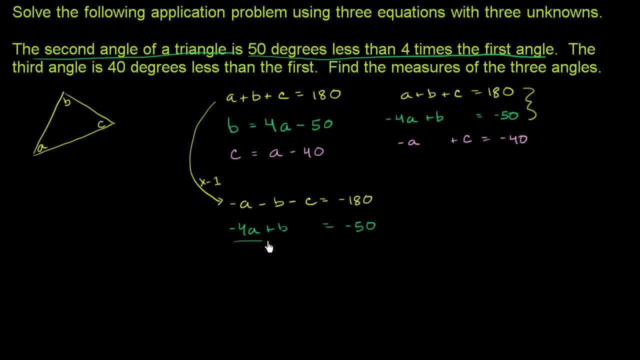 This B is equal to negative 50.. We can add these two up now And we get negative. A minus 4A is negative 5A. The B's cancel out. We have a minus C is equal to negative 180 minus 50. 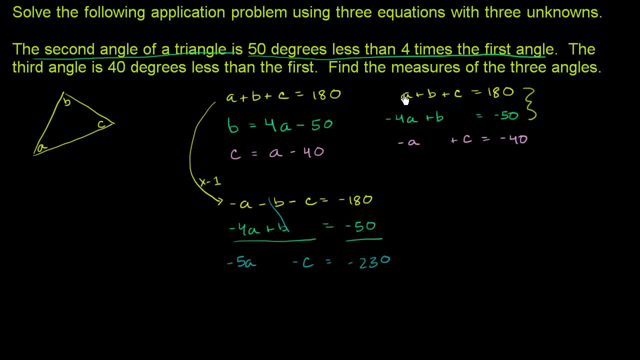 is negative 230.. So now, using these top two equations, we have an equation only in terms of A and C. We have another equation only in terms of A and C, And it looks like if we add them together, the C's will cancel out. 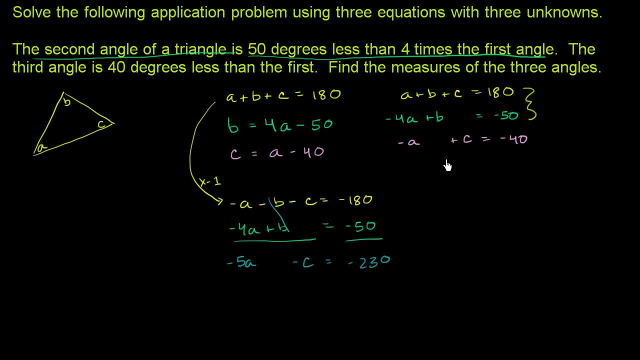 So let me just Rewrite this equation over here, And you have to be careful that you're using all of the equations, Otherwise you'll kind of do a circular argument. You have to be careful that over here this first equation came from these two over here. 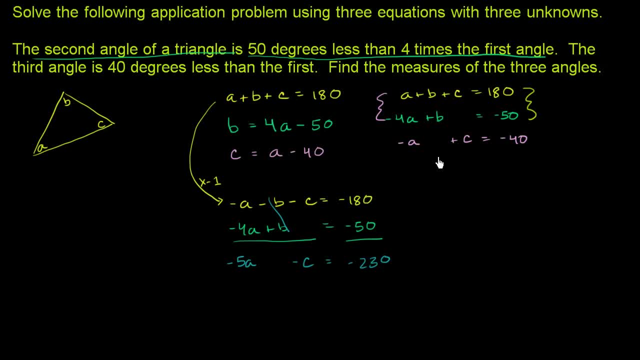 Now I want to combine that with this third constraint, a constraint that's not already baked into this equation right over here. So we have: negative A plus C is equal to negative 40. And we add these two equations- Negative 5A minus A- is negative 60. 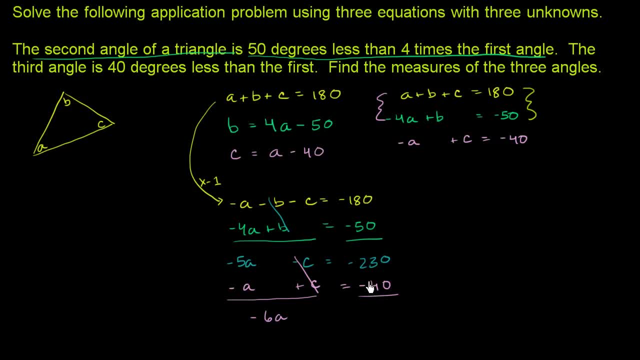 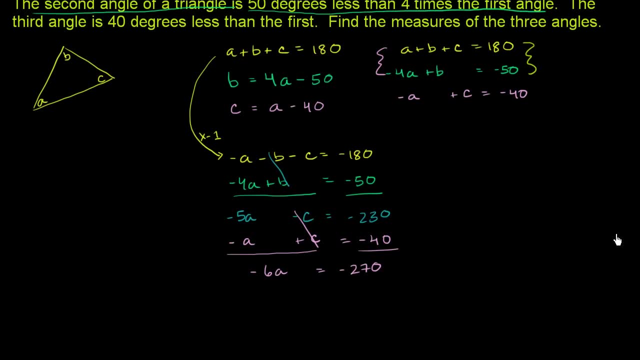 Let's say The C's cancel out And then you have negative 230 minus 40. This is equal to negative 270.. We can divide both sides by negative 6. And we get A is equal to negative 270 over 6.. 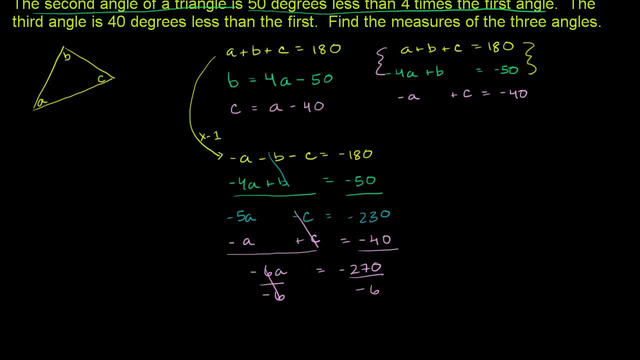 Let me see how many times. Let me see something: 270 is divisible by both 3 and 2.. So it should be divisible by 6.. So let me just divide it: The negative 270.. Negative signs: Obviously a negative divided by a negative. 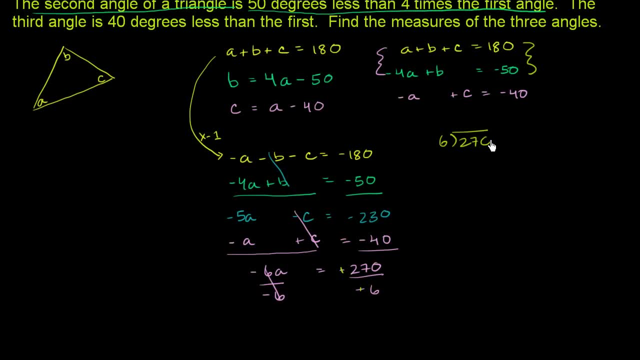 is going to be a positive. And if we take 6 into 270,, 6 goes into 27 four times. 4 times 6 is 24.. We subtract, We get 3.. Bring down the 0.. 6 goes into 30 five times. 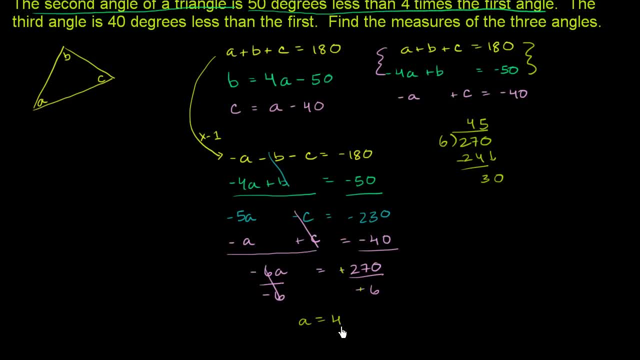 So we get: A is equal to 45.. Now let's look at the other ones We can substitute back in to solve for C. C is equal to A minus 40 degrees. So that is equal to. Let me write it right over here in yellow: 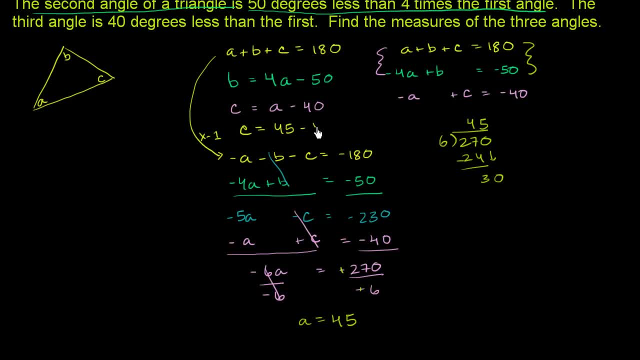 So C is equal to 45 minus 40, which is equal to 5 degrees. So so far we have: A is equal to 45 degrees, C is equal to 5 degrees, And then you could substitute into either one of these other. 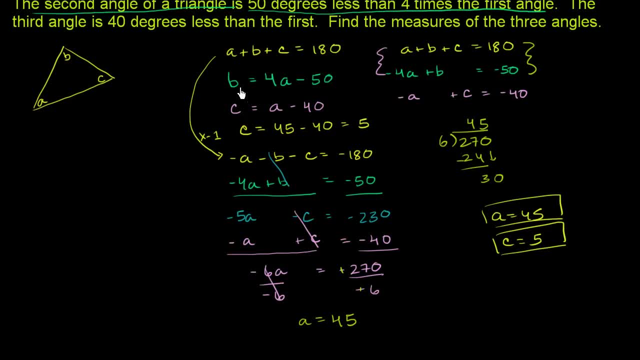 ones to figure out B. We could use this one right over here in green. B is equal to 4A minus 50. So B is going to be equal to 4 times 45 is. let's see: 2 times 45 is 90.. 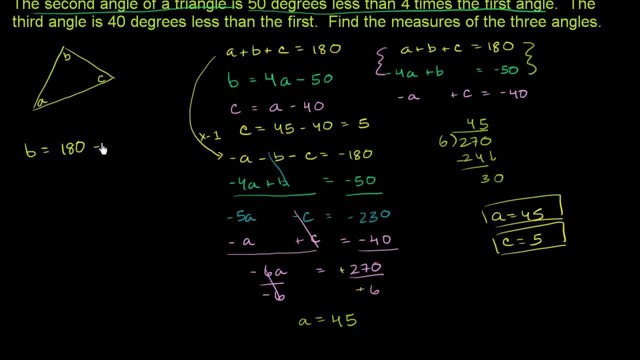 So 4 times 45 is 180.. So it's going to be 180 minus 50 by this equation right over here, which is equal to 130 degrees. So we get: B is equal to 130 degrees, And then we can let me write it over here. 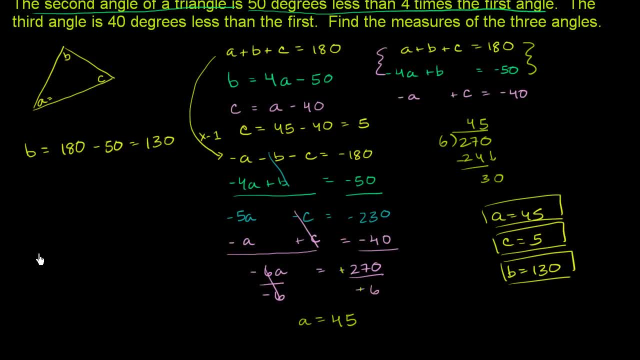 So A is equal to 45. So if I actually were to, if I wanted to draw this triangle, it would actually look something like this: A is a 45 degree angle, B is a 130 degree angle And C is 5.. 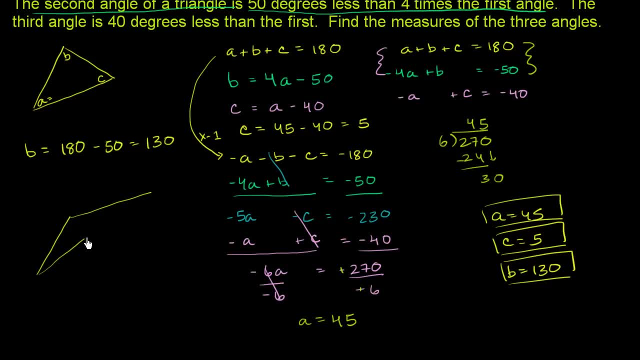 So it'll look something like this. It will look something like this, where this is A at 45 degrees, B is 135 degrees And then C is 5 degrees, And you can verify that it works. One you could just add up the angles. 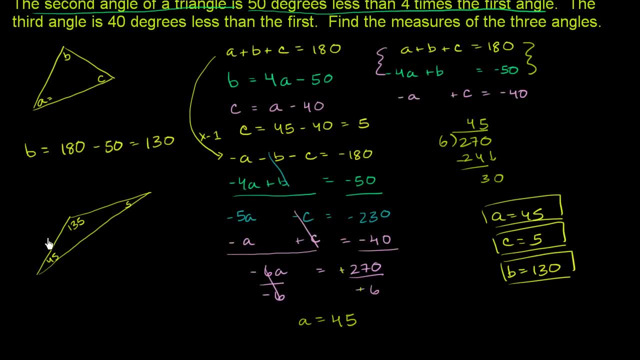 45 plus 5 is 50.. Oh sorry, this isn't 135.. It's 130.. We solved it right over here. It's 130, and this is 5.. So when you add them all up- 45 plus 130 plus 5,- 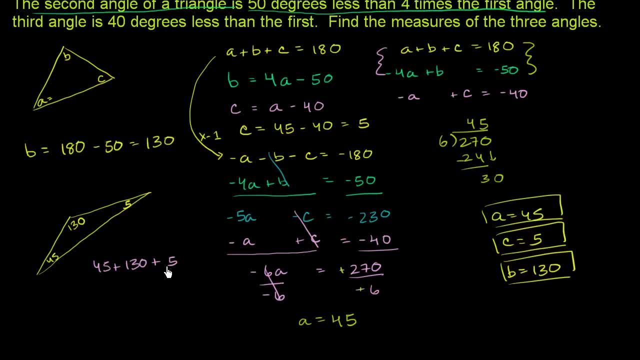 that does indeed equal 180 degrees. 45 plus 5 is 50 plus 130.. So this does definitely equal 180.. So it meets our first constraint. Then, on our second constraint, B needs to be equal to 4A minus 50.. 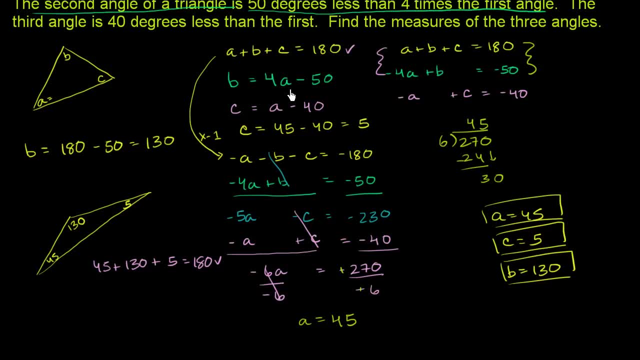 Well, 4 times A is 180.. 4A minus 50 is 130 degrees. So it meets our second constraint. And then our third constraint: C is A minus 40 degrees. Well, A is 45.. C is 5.. 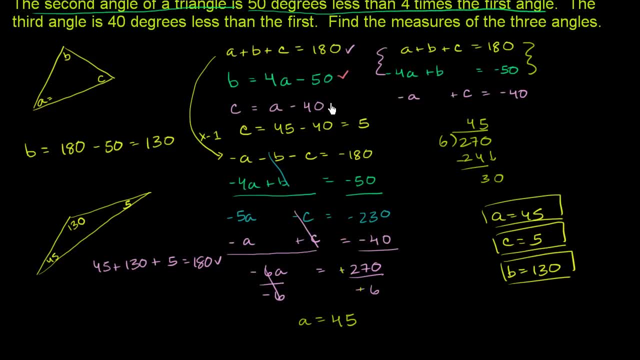 So if you subtract 40 from 45, you get 5, which is C. So it meets all of our constraints and we are done. 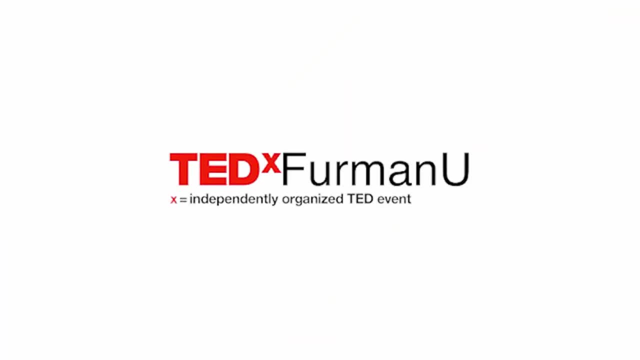 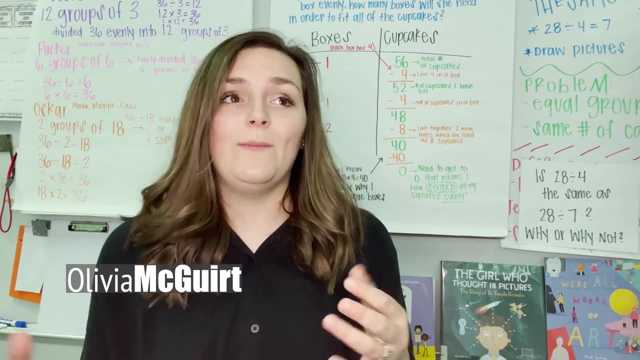 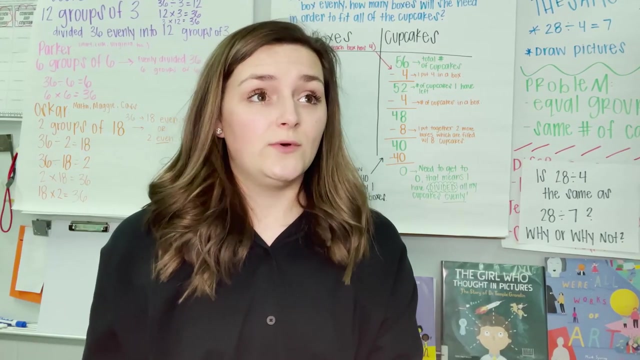 When you were younger, were you ever up really late doing math homework? and it would end in an epic screaming battle about how this is not the way you're supposed to do it. Everyone is red in the face, toughing and puffing and zero gets accomplished. Since we're all virtual, I'm going 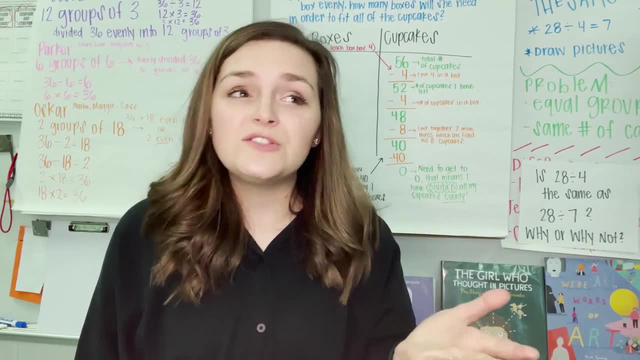 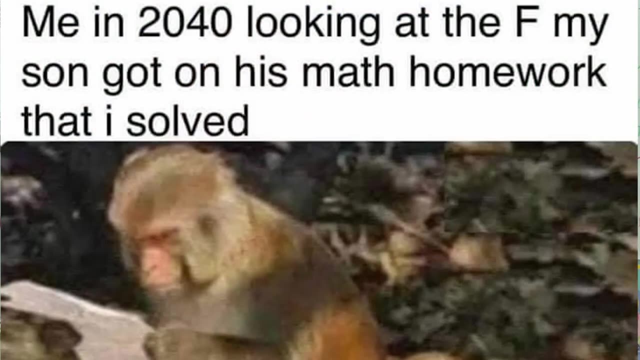 to assume that you all are nodding your heads in agreement with me. So thinking of this reminds me of all the memes I've collected over the last couple years and I want to share a couple with you. So this first one is me in 2040 looking at the F. my kid got on their math homework when I did. 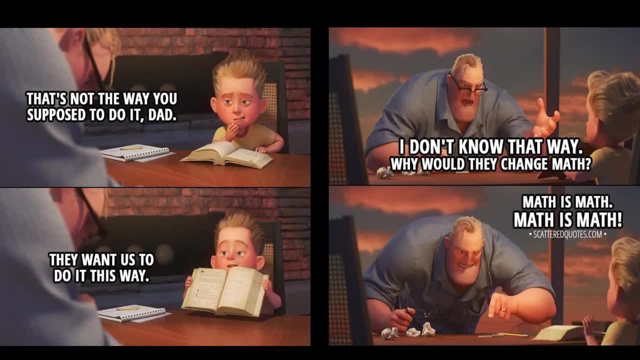 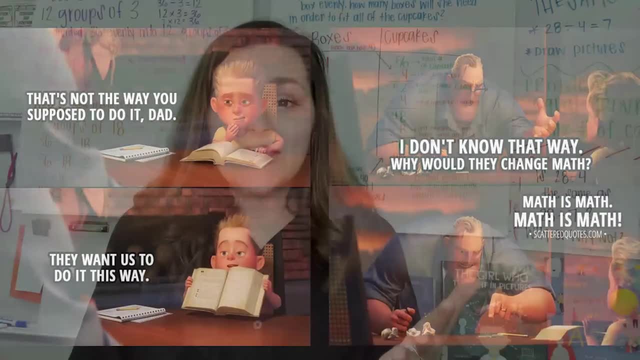 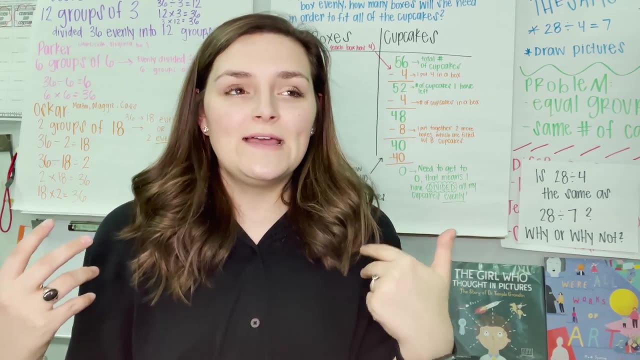 it. And this next one especially reminds me of all the times that my dad and I were at the dining room table doing math, when he would say: math is math, math is math. And so today I want to take you on my journey of what it's like, from when I went from a student to now an educator. So, as a 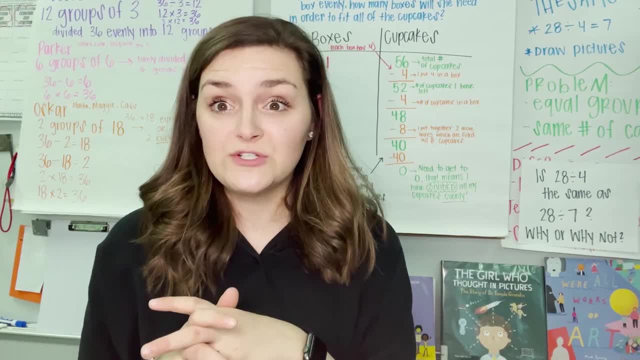 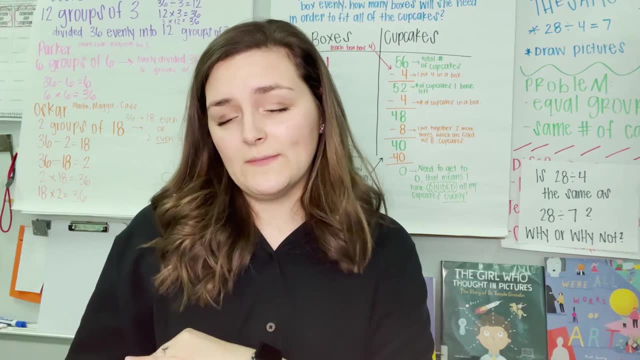 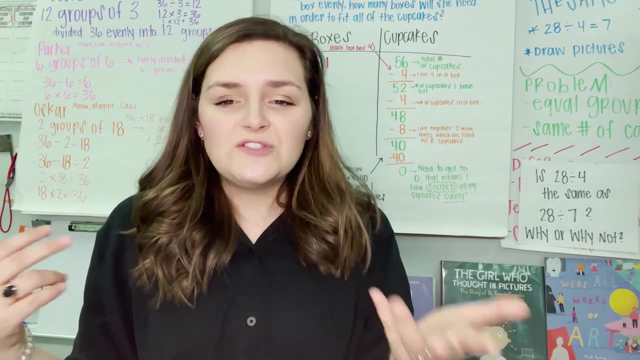 child. I attended an elementary school where I was taught math and science and Spanish for six years and I had a really positive experience with this And I still sometimes, to this day, think about going getting my Spanish certificate so I can go teach at the school. Stay tuned, you may find me there in a couple of years, who knows So but on